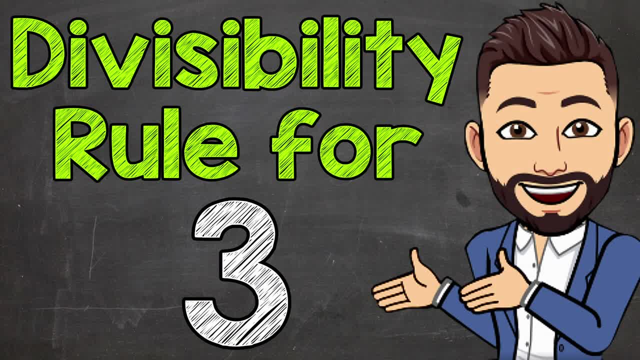 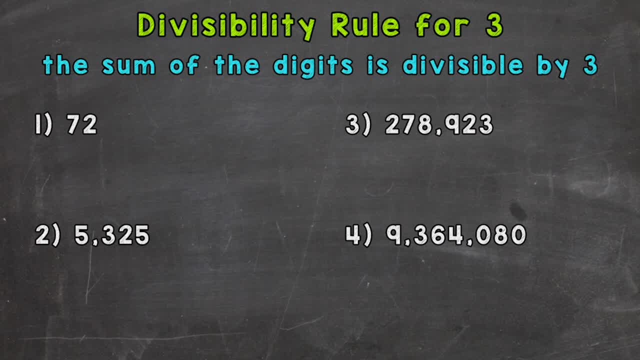 Welcome to Math with Mr J. In this video I'm going to cover the divisibility rule for 3.. Now remember, when we're checking for divisibility, we're checking to see if we can divide without getting a remainder, so the given numbers work out exactly. 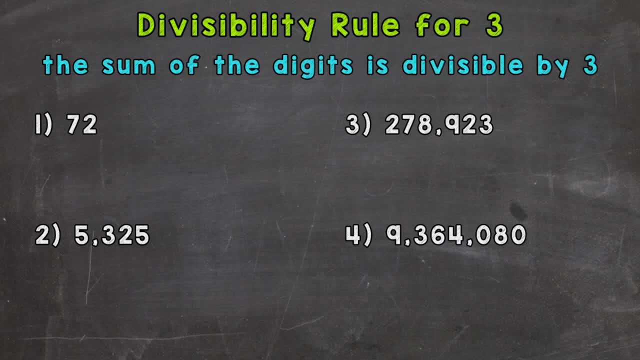 We have four numbers here that we're going to see if they are divisible by 3, based on the rule at the top of the screen. So what we need to do, we need to find the sum of the digits and see if that sum is divisible by 3.. 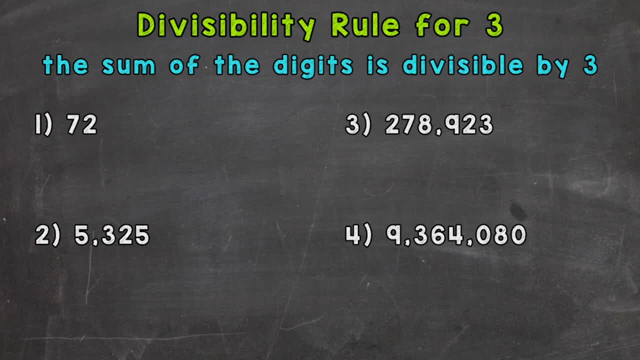 If so, the number is divisible by 3.. Let's jump into number 1 here, where we have 72. So we need to find the sum of the digits. That means we do 7 plus 2. So the 7 plus the 2.. 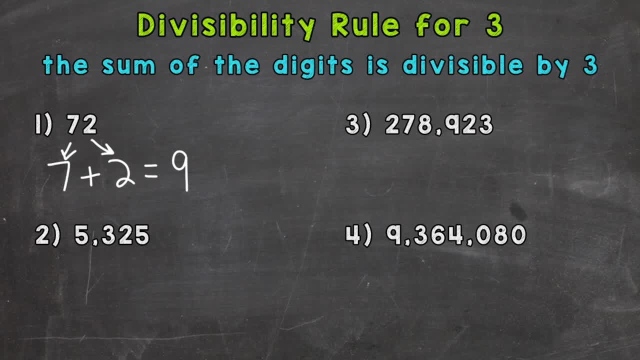 And that gives us 9.. So we need to see if that sum is divisible by 3.. Okay, Can we do 9?? We can do 9 divided by 3 and get an answer that doesn't have a remainder. Yes. 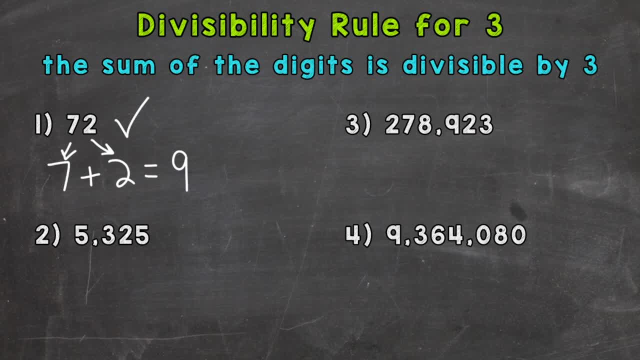 So that means 72 is divisible by 3.. On to number 2, where we have 5,325.. Let's find the sum of those digits. So 5 plus 3 plus 2 plus 5.. So 5 plus 3 is 8 plus 2 is 10 plus 5.. 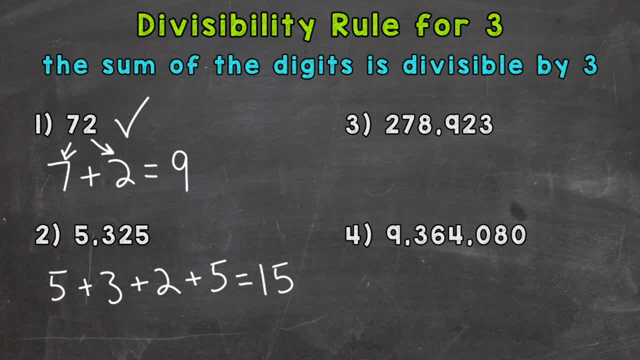 So 5 plus 3 plus 2 plus 5 gives us 15.. So is 15 divisible by 3? Can we do 15 divided by 3 and get an answer without a remainder? Yes, we get 5.. So that means our original number- 5,325, is divisible by 3.. 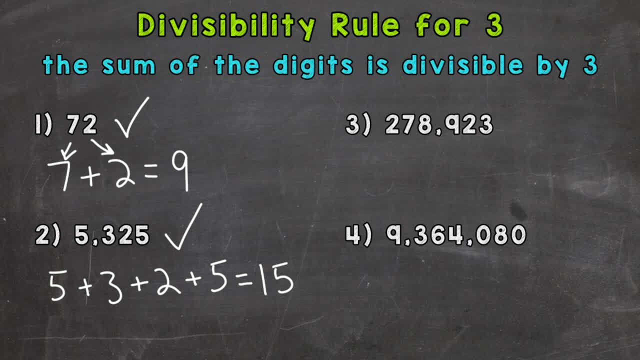 On to number 3, where we have 278,923.. Let's find the sum here: 2 plus 7 plus 8.. Plus 9 plus 2 plus 3.. So that gives us 2 plus 7 is 9.. 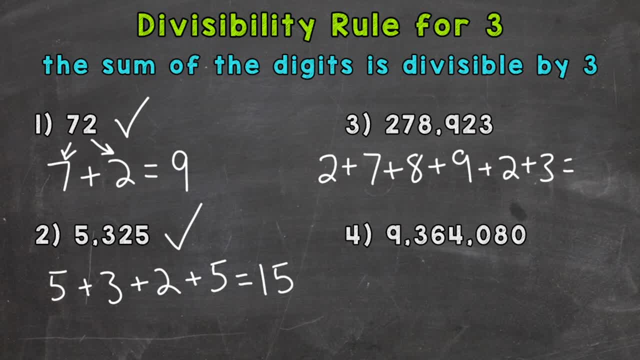 Plus 8 is 17.. Plus 9 is 26.. Plus 2 is 28.. Plus 3 is 31.. Now, 31 is not divisible by 3. We get a remainder with that answer. So again: 31 not divisible by 3..